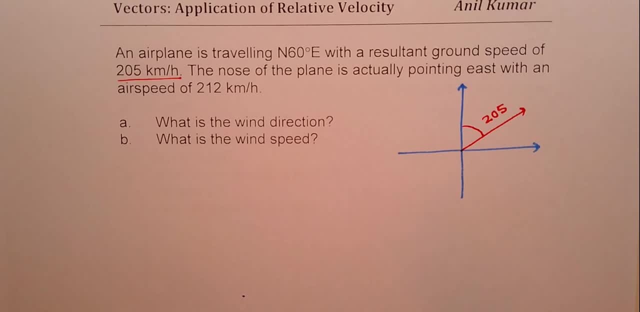 Now we are also given that the nose of the plane is actually pointing east with an airspeed of 212. So let us say 212 is slightly longer. So let's say kind of like this: So pointing east, that means the plane is going towards east but because of wind it moves in. 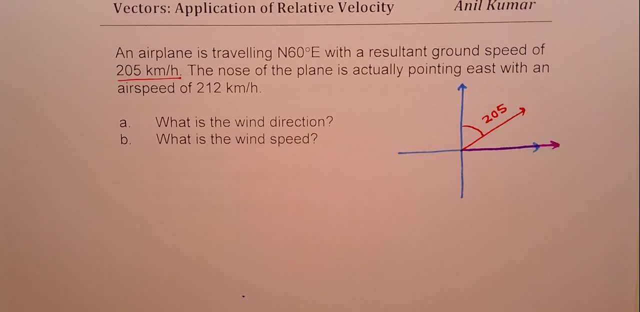 that direction You get an idea right. So the resultant is as shown in orange And that is because of the wind right. So it says: what is the wind direction? So wind direction is something like this. Now I hope the diagram is clear. that is called the vector diagram. We. 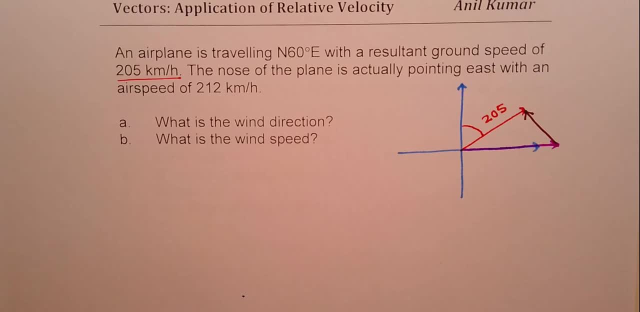 need to find the wind direction and the when speed. Now this angle here is 60 degrees and this will be 30 degrees. Total is 90 degrees. Here we are considering north- No plane actually is going in towards south- and then we are going to rise north and then we are going into north. It is what we are discovering here. So now we are observing this north side and we are going back north through east, So this crew that is seen as the right side, and then we are aligning north one to east. conditions like this, As far as we can see, it's not that different. 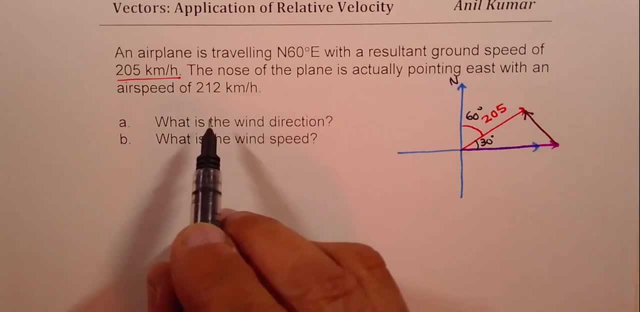 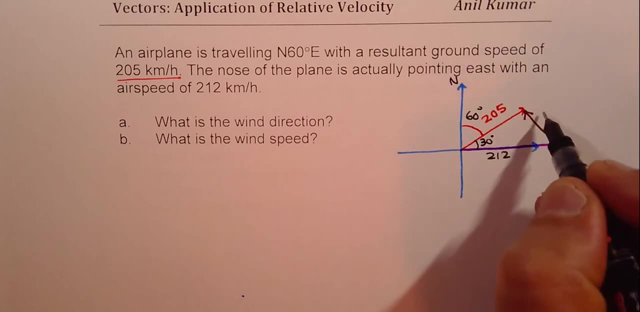 towards East at a speed of 212 kilometers per hour. But because of the wind- let's say wind velocity- the resultant is 60 degrees East of North. Is that clear? So what you see here is a right triangle where two sides and an angle included is given. 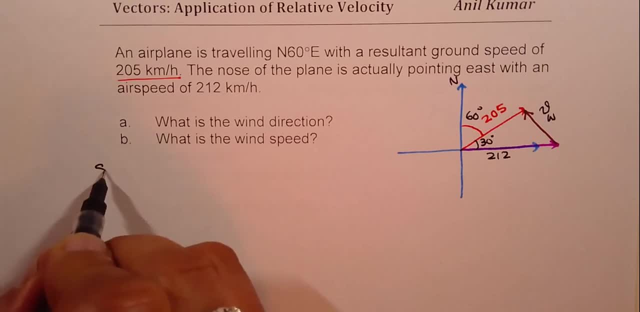 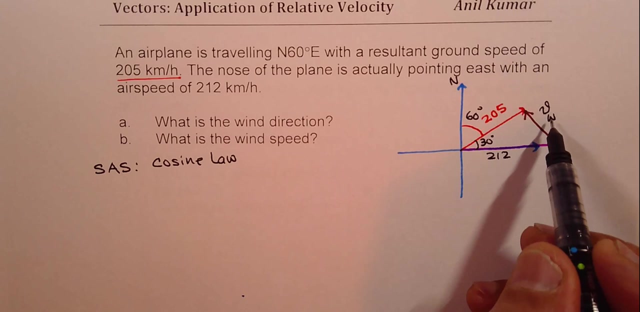 So what we have here is side, angle side, and that means you can apply cosine law. Is that clear? So, applying cosine law, we can find the wind velocity. So wind velocity is equal to: let me write down: square of. this is equal to square of. 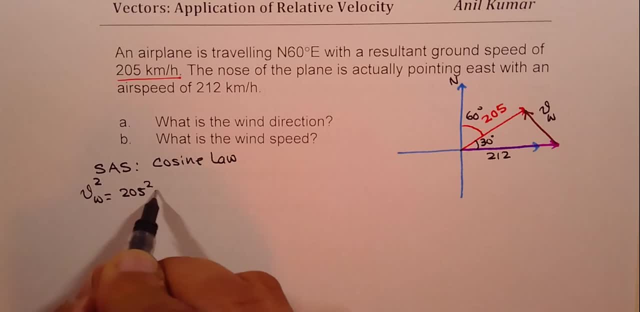 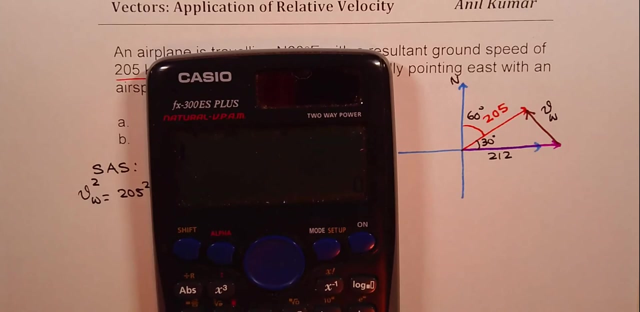 205 plus square of 212.. Minus 2 times 205, times 202, times cos of angle 30 degrees, So you get angle 30 degrees, which it makes with the East. Now let's calculate this. So first our calculator should be in degrees. 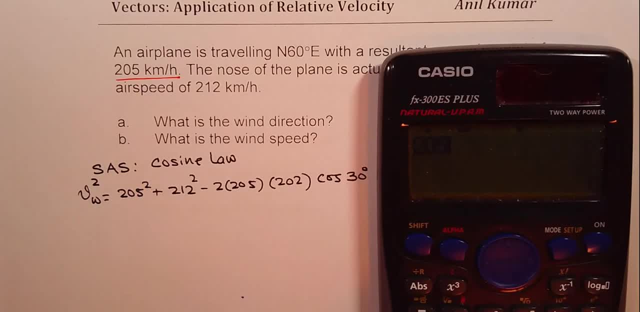 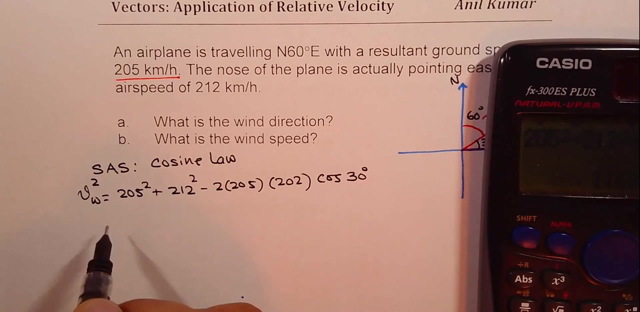 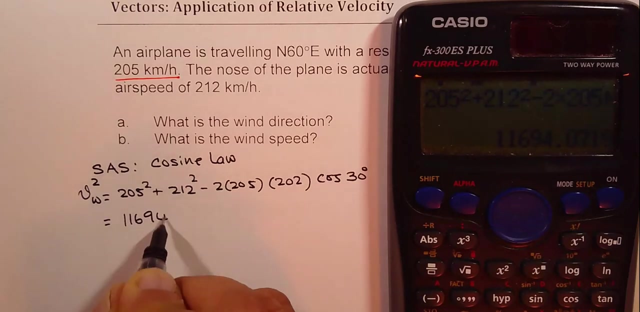 And now let's calculate this answer: 205 squared plus 212 squared Minus 2 times 205 times 212 times cos of 30 degrees, Is equal to a big number, which is 11694, 11694.. So we'll do the square root of this to get wind velocity. 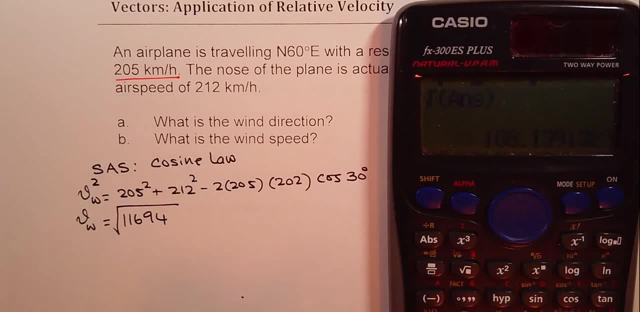 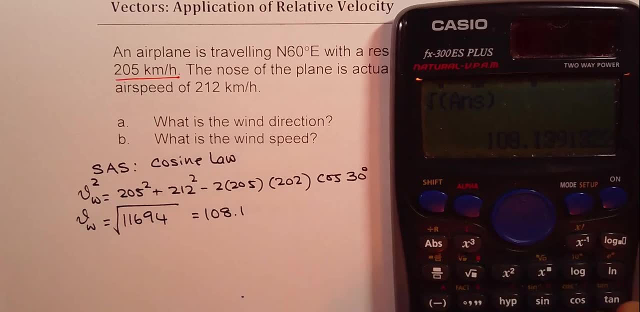 Let's find square root of our answer, which is 108.13.. So we get 108.13.. Okay, Okay, So we got 108.13. point. let's say one: The units are kilometers per hour, Is that clear? 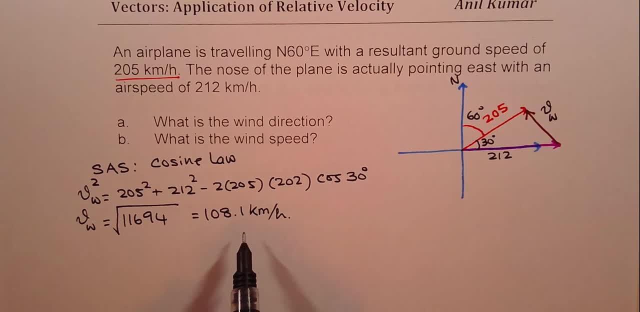 So we got the wind velocity. Now we need to find the direction. So once you know wind velocity, you can actually find the direction using sign. So for the direction, let's find this angle first and then we'll work out, Okay. 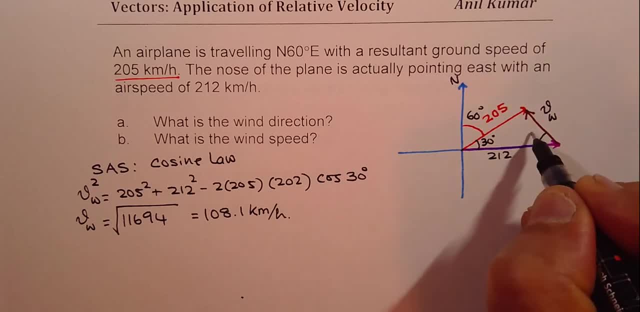 We have this angle, So let's call this direction as theta. so in that case, sine theta over 205 is equal to what we calculated. wind velocity of We'll write in denominator wind velocity of 108.1 over the angle of 30 degrees, sine of 30 degrees. 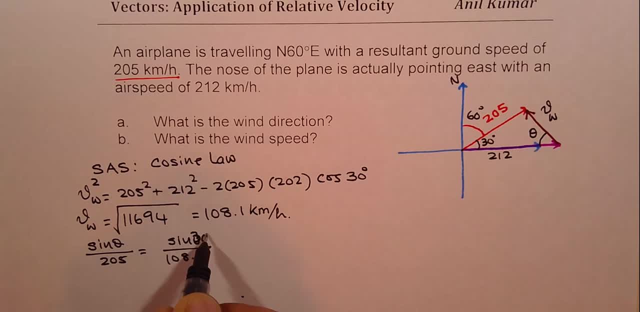 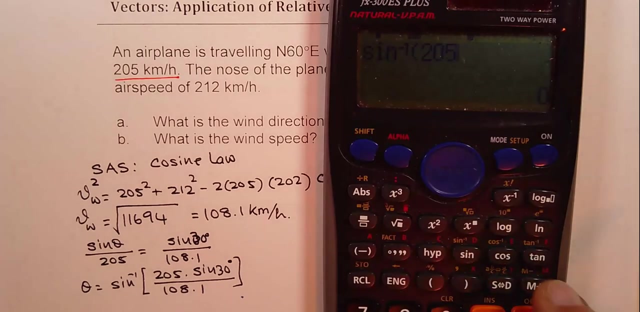 of Correct. so from here We can find what theta is. so we can say: theta is sine inverse of 205 times sine of 30 degrees divided by 108.1. So let's find this, so we'll do shift: sine inverse of 205 times. 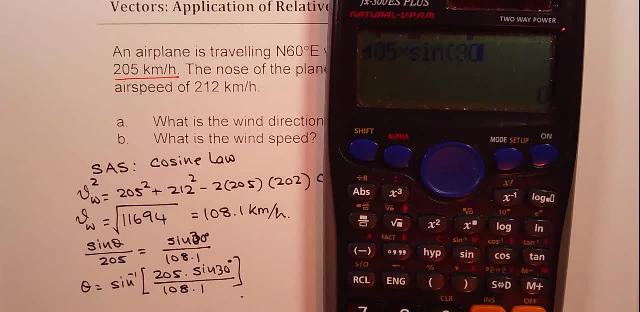 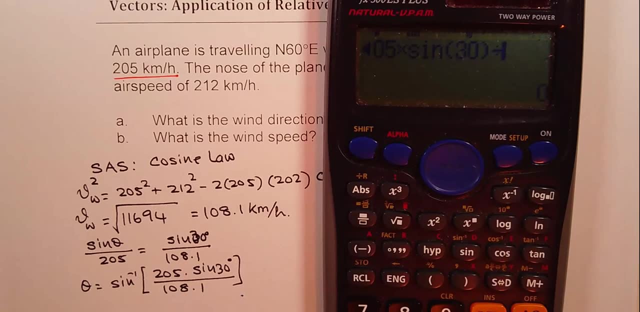 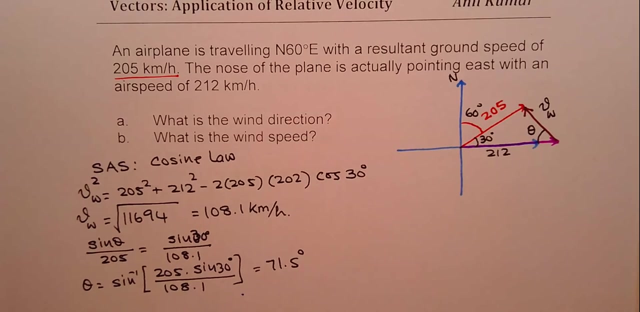 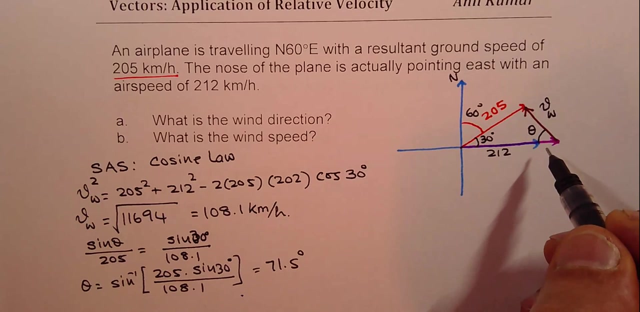 sine of 30 degrees divided by 108.1 bracket, close equal to, So we get seventy one point four, seven, So we get seventy one point. Let's say five degrees. This angle is seventy one point five degrees. now, how to describe this angle? Now, you could describe this angle in many different ways. 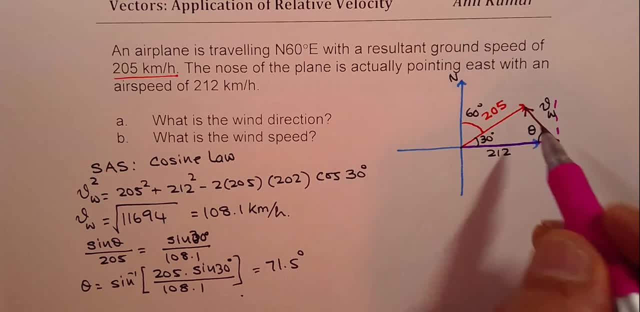 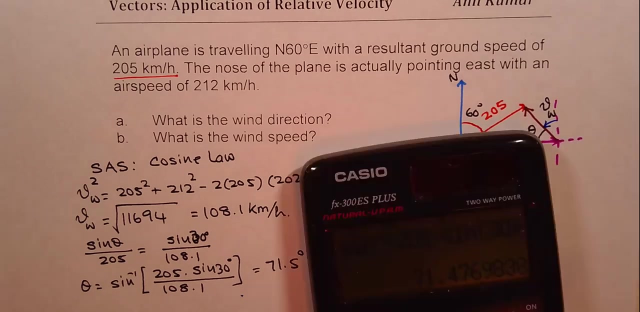 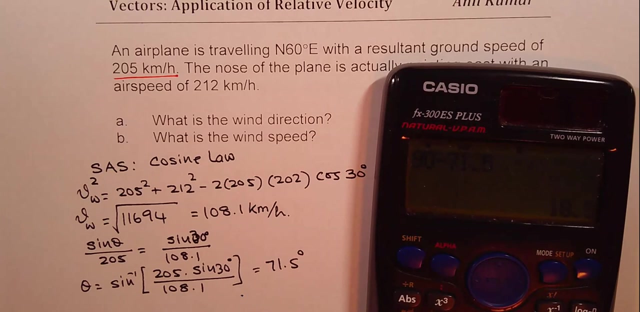 Let's say that is the north right, So, and this is East, So you could say that this angle is From North. How many degrees West? All right, so that you could do so, we could say 90 minus seventy one point five, ninety minus seventy one point five, which gives you eighteen point five degrees. 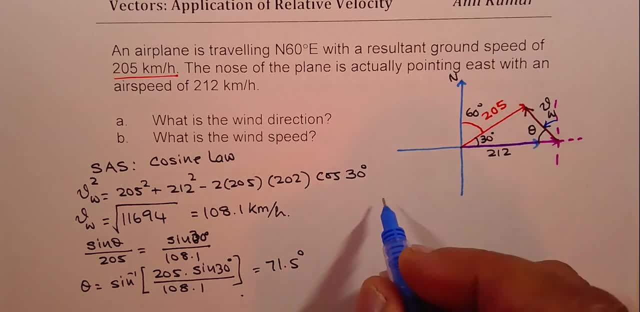 so this could be, so we can say wind velocity or wind direction Is from North. We have seventy one point five here, so that one which we got, Whether we are getting some wind here. so that means here is 180 degrees West and this is 18.5 degrees West. 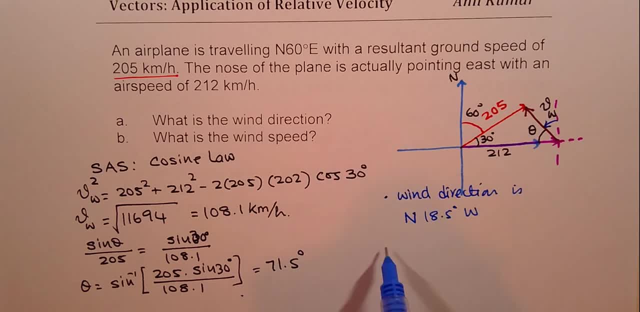 So that becomes the wind direction and we know wind velocity is, and we know wind velocity is velocity hundred and eight point 11 Km poor. So I hope the concept is absolutely clear. so our得원 product is absolutely clear. Fee theory or model competition generatingmanas jobs of the UK. produce in the United States. increase. Lot 설명: 1: 0 to 300.4 ns. This drops directly to lightened hexatons, or meg Nasıl s? can you read about how to write an exercise which isn't exactly the same as the exact flags in 2015? 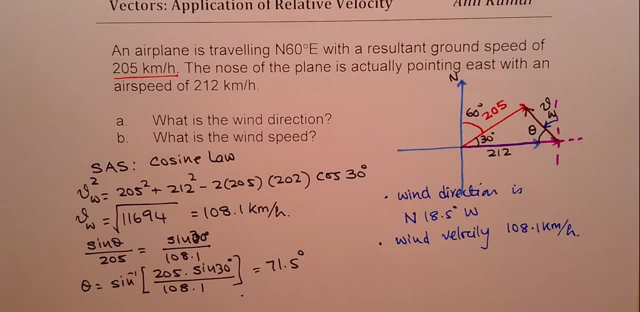 to write your comments, share your views and, if you like, and subscribe my videos. that would be great. Thanks a lot for watching.